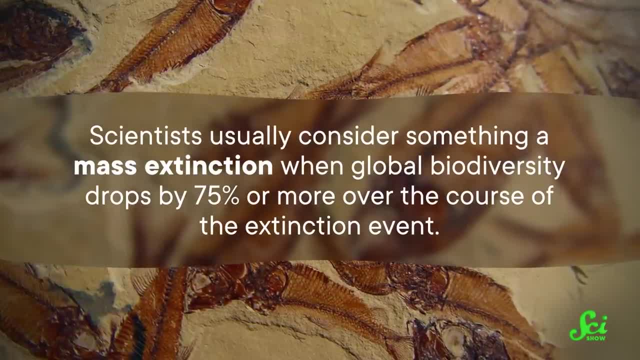 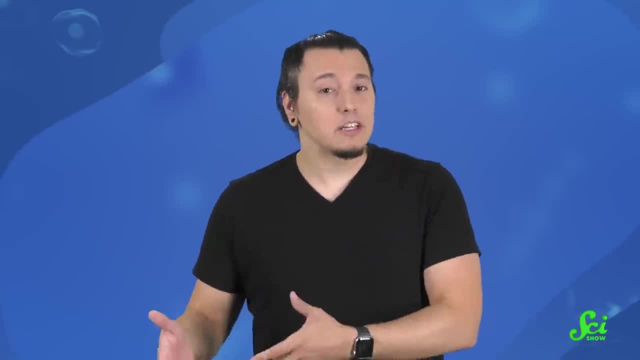 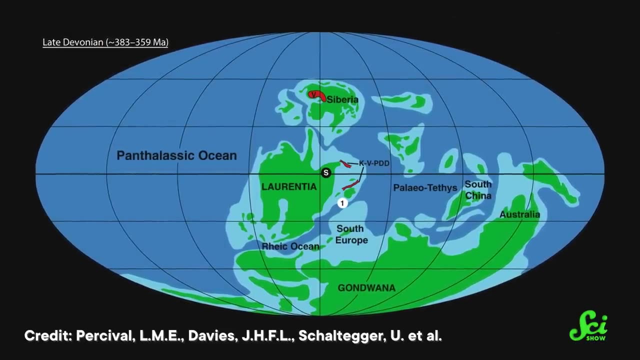 Scientists usually consider something a mass extinction when global biodiversity drops by 75% or more over the course of the extinction event. So the number of species on Earth seriously tanks And the Late Devonian Extinction definitely meets that criteria. This event happened from 375 to 359 million years ago. 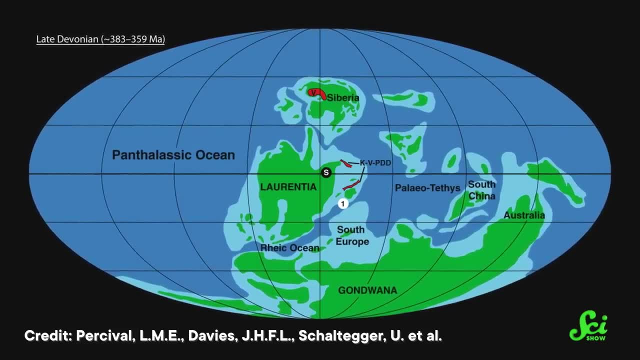 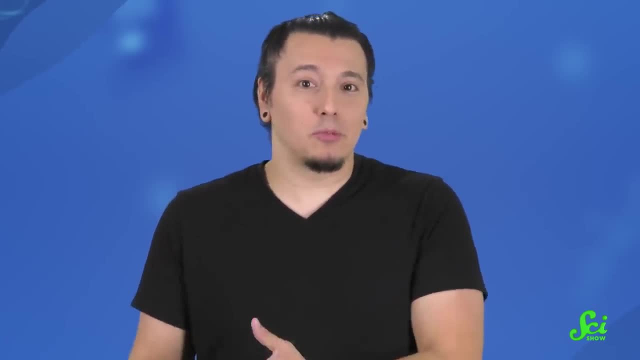 So about 16 million years total, And scientists are still working out exactly how it unfolded. In a typical mass extinction scenario, you'd usually picture mass extinctions, As in lots more things than normal going extinct all at once, But in the Late Devonian it's possible that instead of more things dying out fewer. 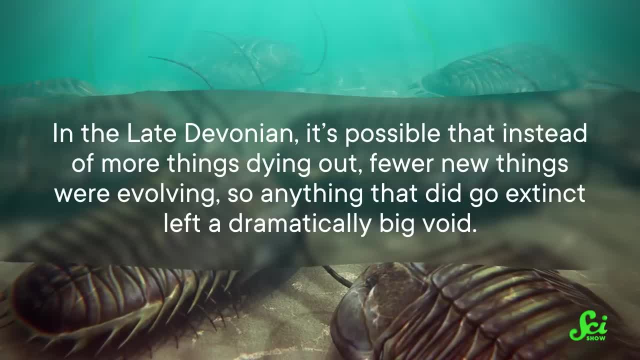 new things were evolving, so anything that did go extinct left a dramatically big void. In any case, they do know that the number of species that are going extinct is going to increase. That's why the number of species on Earth started to tumble, and it didn't stop tumbling. 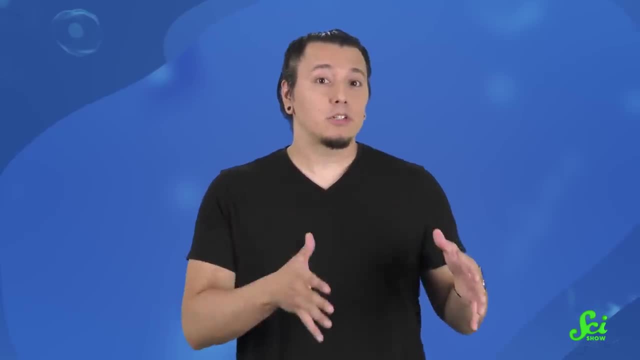 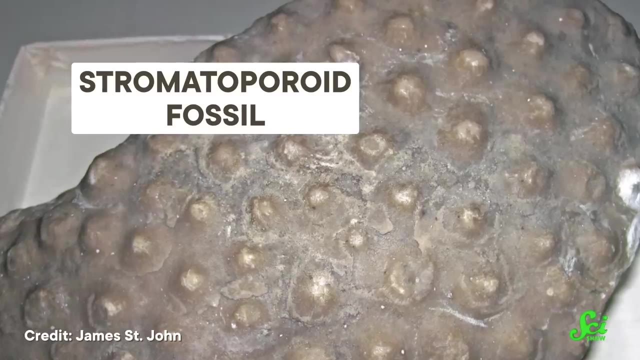 until the very end of the Devonian. In particular, this crash hit ocean ecosystems hard. Animals like stromatoperoids, which were reef-building sponges, disappeared completely, as did the shelled animals that depended on these ecosystems. Our friends the trilobites suffered major losses in the Late Devonian too. 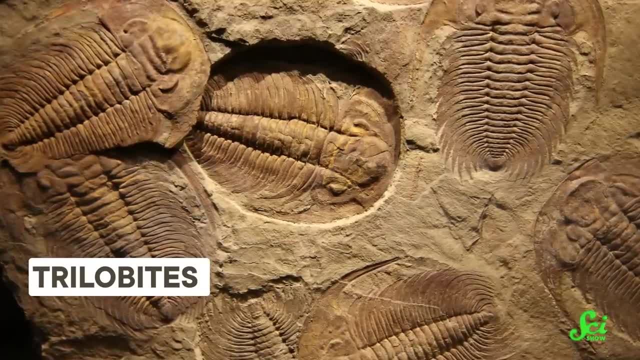 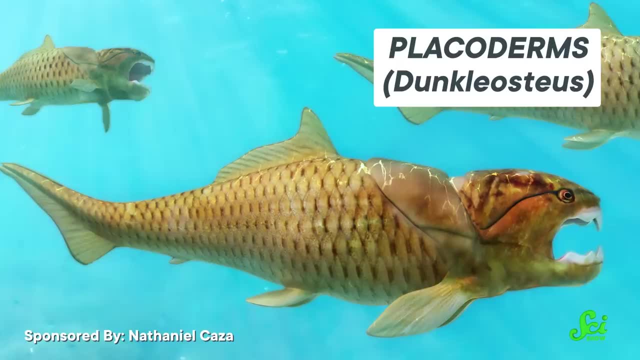 Only one group survived, and they never returned to their pre-Devonian glory. Armor-headed fishes called placoderms were also seriously affected. Here, only two species made it through the extinction, But they were still alive. They survived the extinction event and even they went extinct not long after. 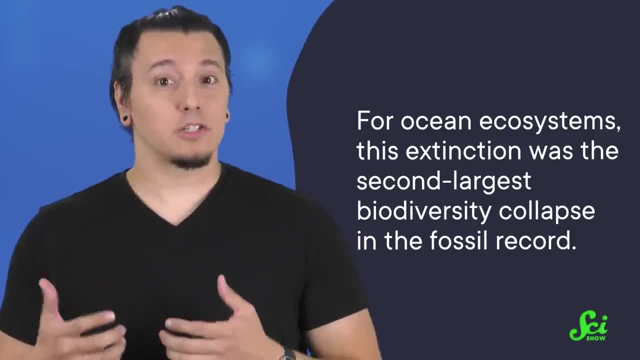 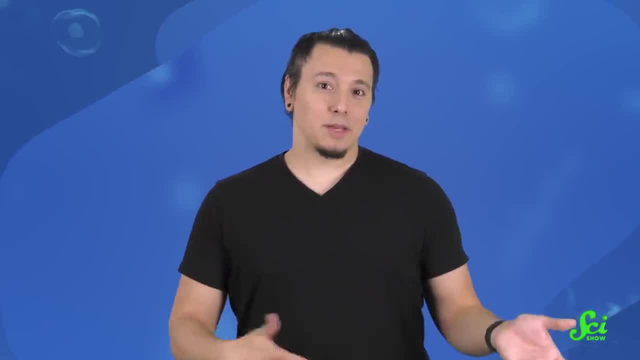 Overall. for ocean ecosystems, this extinction was the second-largest biodiversity collapse in the fossil record. Meanwhile, ecosystems on land were pretty much fine, Like they threw down a big ol' skip card in Uno. so what gives? Well, the reason life on land wasn't as affected by this extinction event might be. 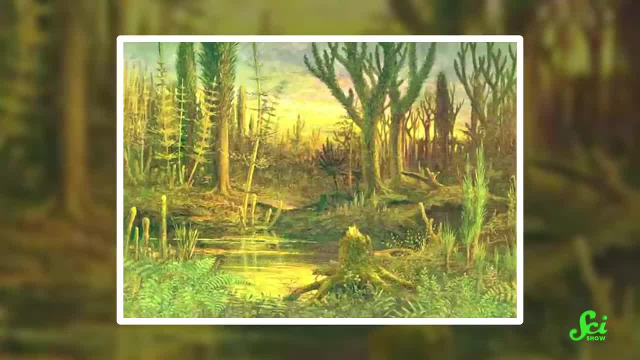 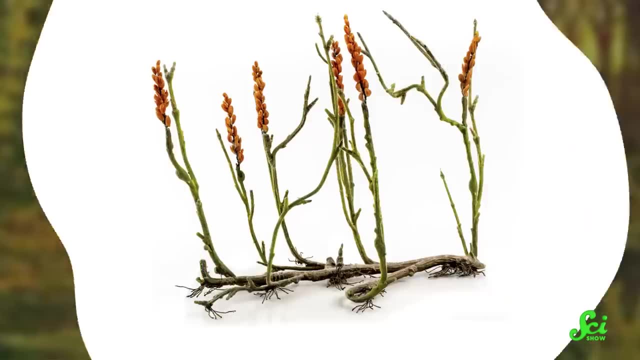 because the organisms living on land were the ones that caused it. Specifically, the culprit may have been trees, which were beginning to evolve around this time, See before this extinction event. land plants weren't very diverse. They were dependent on bodies of water for reproduction, so they couldn't live far. 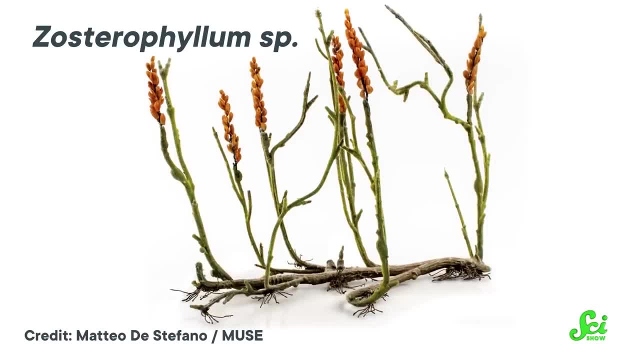 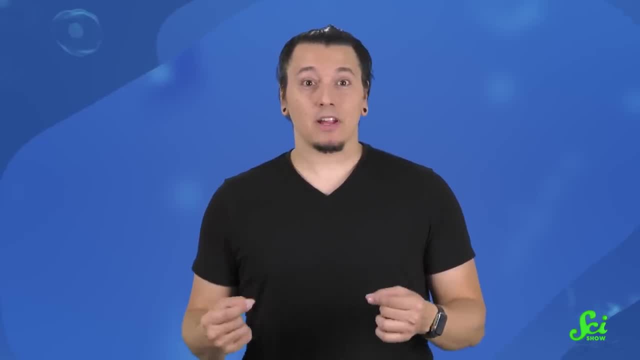 from shorelines, And they weren't very good at moving water around their little plant bodies, so their stems couldn't get very tall, That is until trees evolved. Trees are kind of like the crabs of the plant world. Lots of different kinds of plants keep evolving into tree shapes. 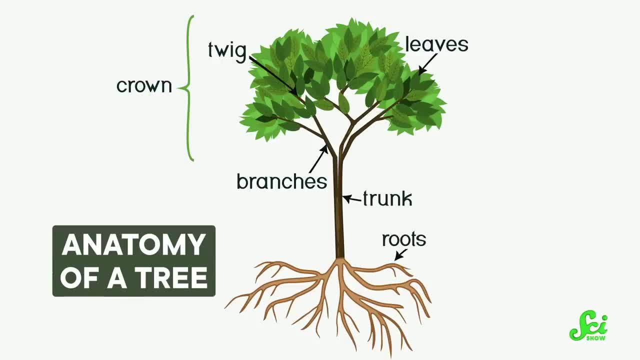 It's a strategy, not a family group. What makes a tree a tree is, very basically, having sturdy, thick stalks or trunks and really strong root systems that can reach deeper water sources and break up sediment as they grow into the Earth. That's why they're so important. When plants figured out how to get big like this, they also started forming seeds with hard shells. These seeds retained water, so the baby plants inside could stay viable far from rivers and oceans. Being big and watertight now meant plants could go a lot of new places. So, all of a sudden, these plants start showing up in the fossil record all over the place, And these Devonian forests may have been bad news for the life in the oceans for two reasons. The first is that their deep roots could have churned up layers of sediment releasing minerals. that used to be bound up in rock. The roots themselves would also help. The roots themselves would also host nitrogen-fixing bacteria, which turn regular nitrogen from the air into compounds that plants can use, like nitrates and ammonia. Those minerals and compounds would have soaked into the water supply and been carried away. 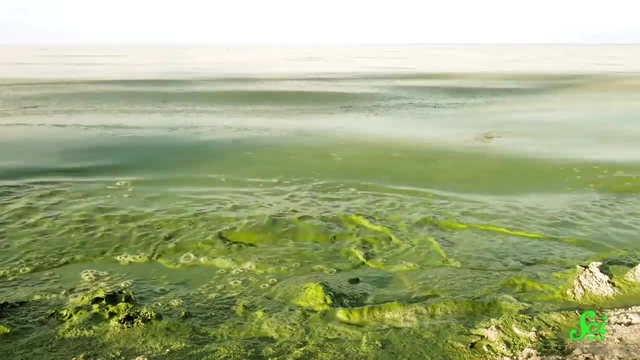 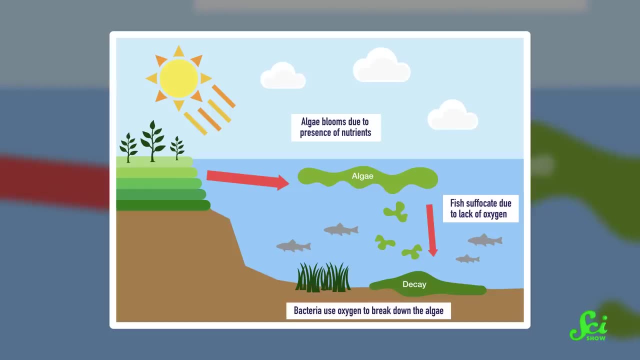 by things like streams, melting snow and rainwater, And when they'd inevitably end up in the ocean, they would have caused an explosive growth of algae. Except those booming algae populations wouldn't have been sustainable, so thick mats of dead plant matter would have soon fallen to the ocean floor all at once- too quickly to be. 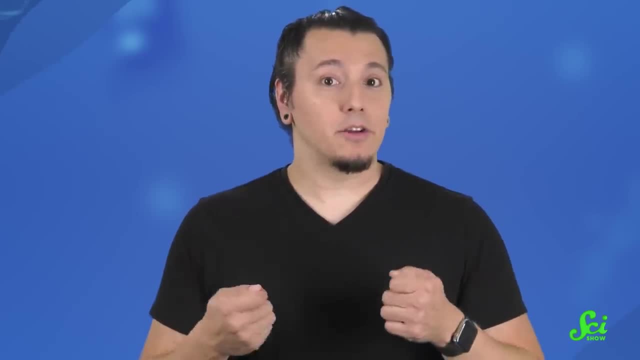 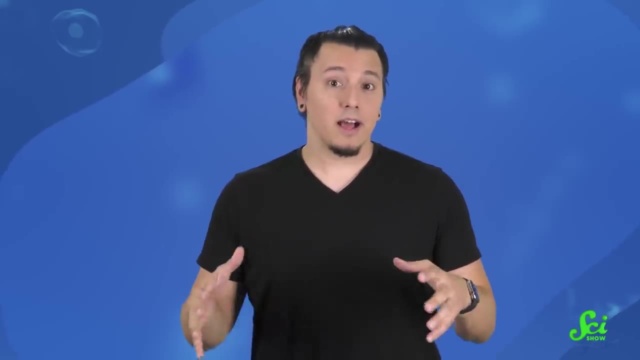 decomposed And they would have basically choked out anything living underneath them. And there go the trilobites. We have evidence that this happened during the late Devonian extinction too. These mats of dead algae produced layers at the bottom of the ocean with basically no oxygen in them, and these layers eventually fossilized into rock. But that isn't the only clue we have leading back to our leafy friends. Big plants also photosynthesize more, and the first trees would have been sucking so much carbon dioxide out of the air that the amount of it in the atmosphere would have plummeted. And since less carbon dioxide means less heat trapped in the atmosphere, this meant that the planet would have cooled down, which we also have evidence for. In fact, the average temperature during the late Devonian extinction dropped between 3 and 6 degrees Celsius, which would have made the ocean way too cold for some marine organisms. 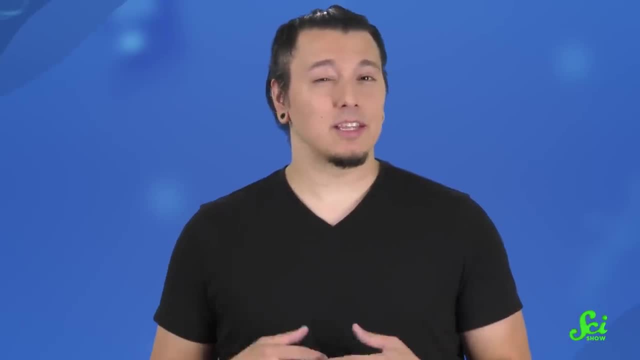 to deal with Now. the tricky thing about both these lines of evidence is that they seem compelling, But neither of them tells us that trees caused this extinction. for sure, Technically, something else could have caused the algae to bloom and die, or the global temperature. 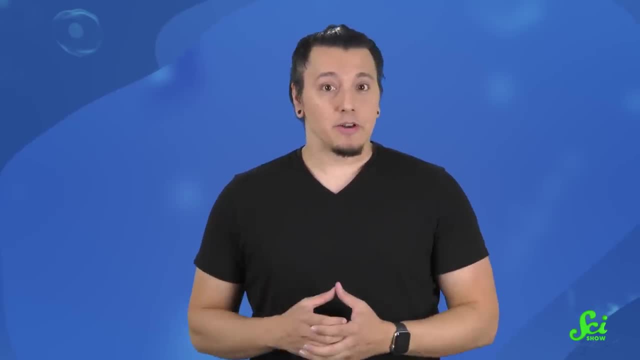 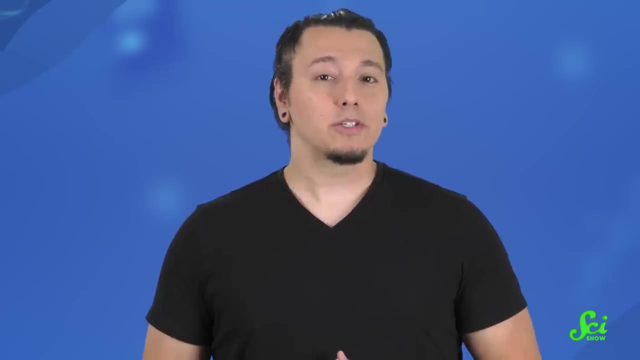 to drop. So some scientists favor other ideas about the late Devonian. from meteor impacts to volcanic eruptions, And unless we find a fossil tree holding a literal smoking gun. the research community may never all agree what happened, But even if they weren't, the main cause of the late Devonian extinction, trees were 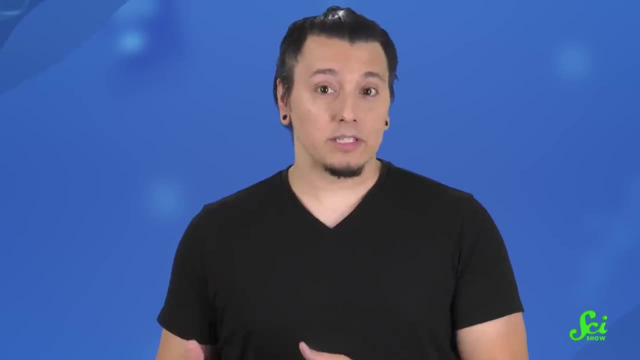 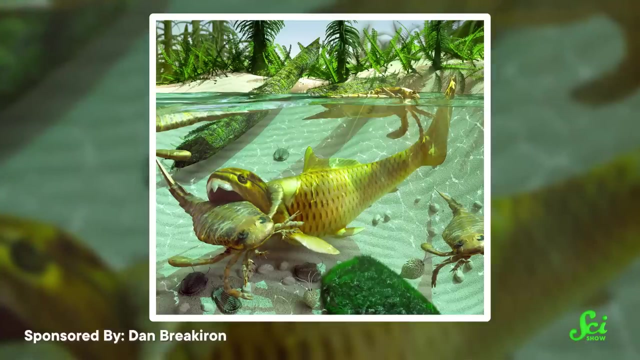 probably playing some role in it. That means the success of one kind of organism likely resulted in the collapse of other ecosystems, Game of Thrones style. So, ultimately, the late Devonian extinction is a great reminder that all life is connected, for better and for worse. 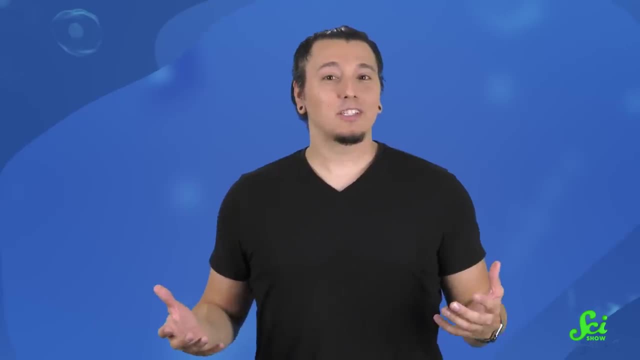 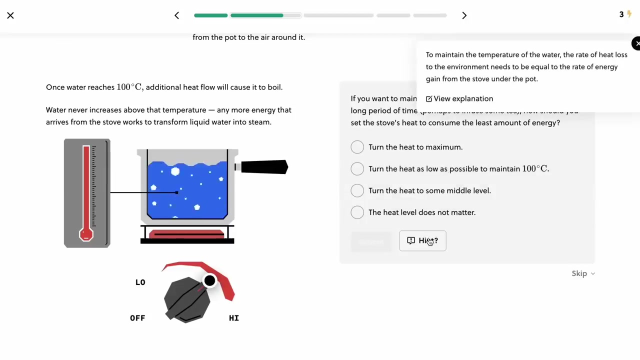 And as we all grow, we all have shared roots. Thanks for watching this SciShow video and thank you to Brilliant for supporting it. Brilliant is an online learning platform that offers guided, problem-solving-based courses in math, science and engineering. 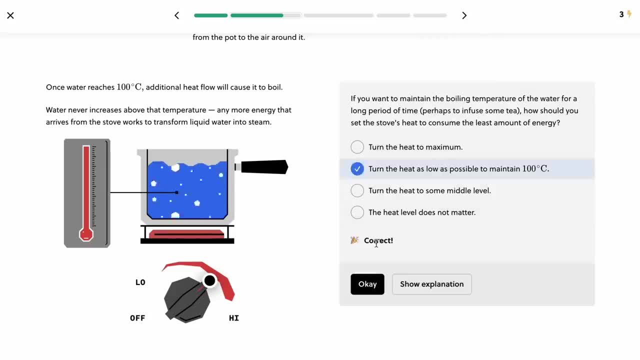 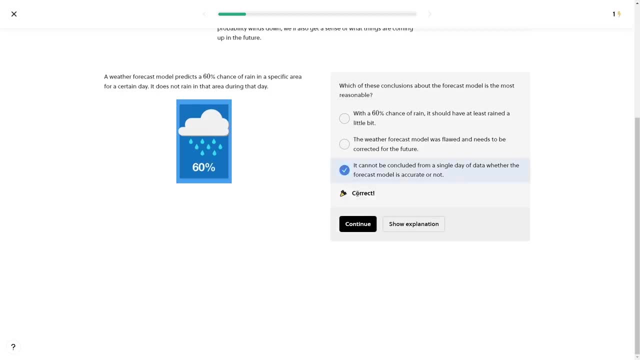 They've supported SciShow for years and we're happy that they're supporting this video as well. With the Brilliant course Applied Probability, you can get the foundation for figuring out the probability of another mass extinction. And that's just one application of probability. 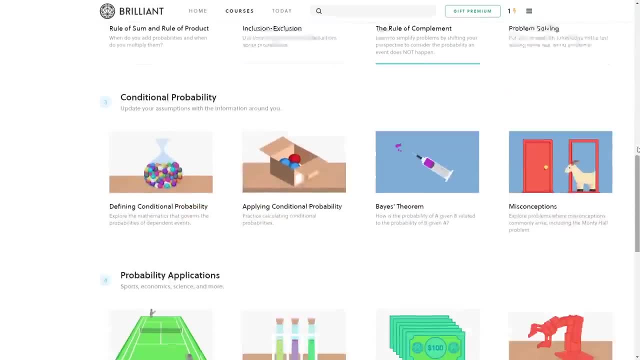 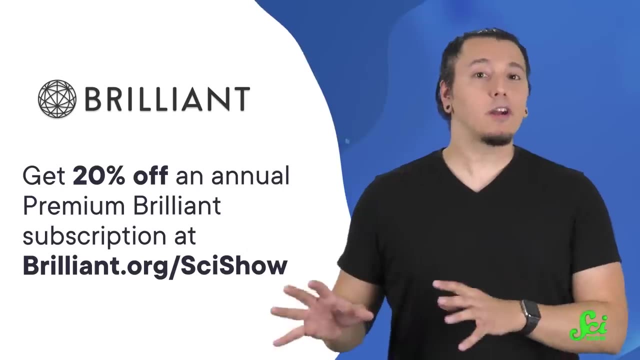 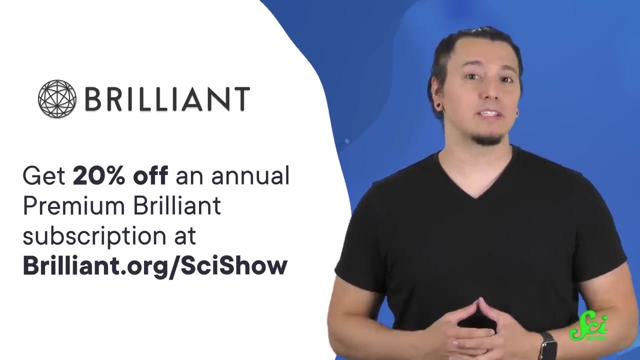 Throughout 23 interactive lessons, you'll explore a variety of circumstances for thinking probabilistically, From astrology to tennis. you can even forecast the financial future. But even before starting this Brilliant course, your financial future is looking up, because the link in the description below will give you 20% off an annual Premium Brilliant subscription. 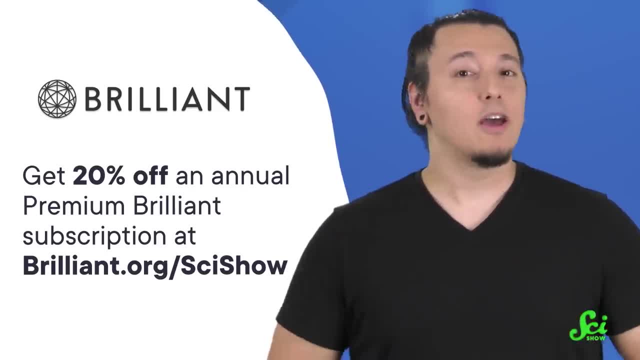 Before you commit to a year of Brilliant, you can try it for free using that link or by visiting Brilliantorg slash SciShow.